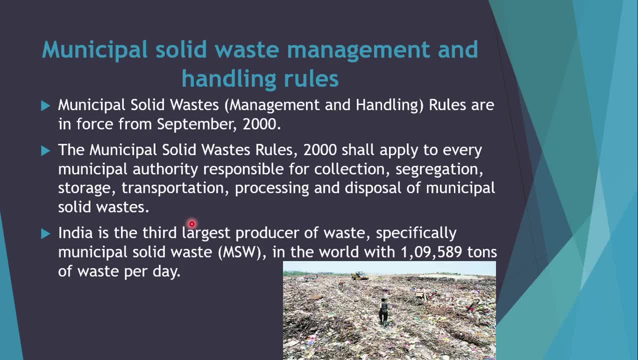 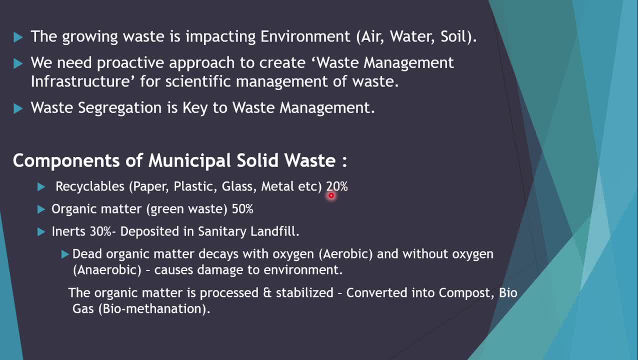 India is the third largest producer of waste, specifically municipal salt waste, in the world, generating a role 20% of municipal solid waste. Next, organic waste. Organic waste can be degradable: It comes around 50% Inerts. that means just the waste has to be thrown in the landfill area. It comes around 30%. 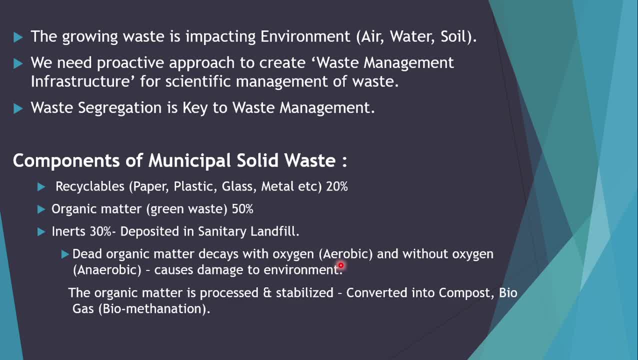 Dead organic matter decays in the presence of oxygen. that means aerobic degradation and also in absence of oxygen, anaerobic degradation causing damage to environment. So the organic matter is processed and stabilized. It can be better converted into compost, vermicompost, biogas and other fuels. 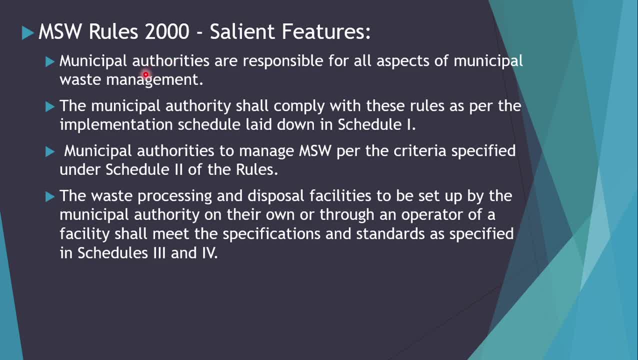 The salient features of organic matter. Municipal authorities are responsible for all aspects of municipal waste management. The municipal authorities shall comply with these rules as per the implementation schedule laid down in Schedule 1.. The municipal authorities to manage municipal solid waste per the criteria specified under Schedule 2 of the rules. 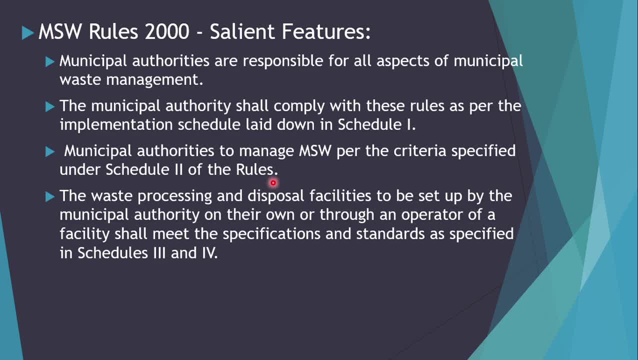 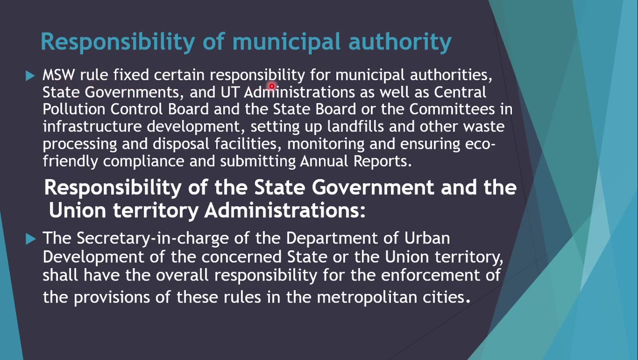 The waste processing. Also, the inventory of the waste facilities shall be the specifications and standard as specified in Schedule 3 and 4.. Cause of indefinite waste management: The Responsibilities of Municipal Authorities. The municipal authorities must contain the responsibilities of municipal authorities and state governments and the union territory administrations, as well as Central Pollution Control Board and the State Board or 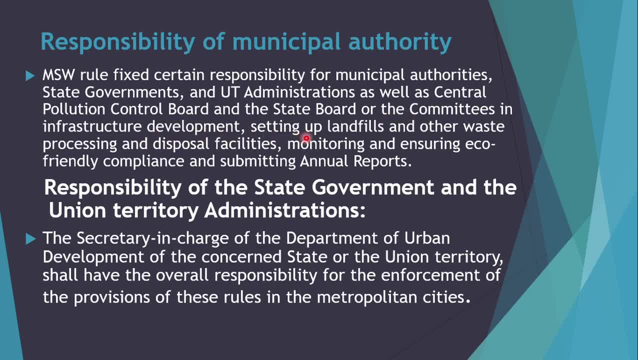 the committees of the PUMI Body, ipanob for electoral data, Alsoрупhpdcom Okay. infrastructure development in setting up landfill areas and other waste processing and disposal facilities, monitoring and ensuring eco-friendly complaints and submitting annual reports. 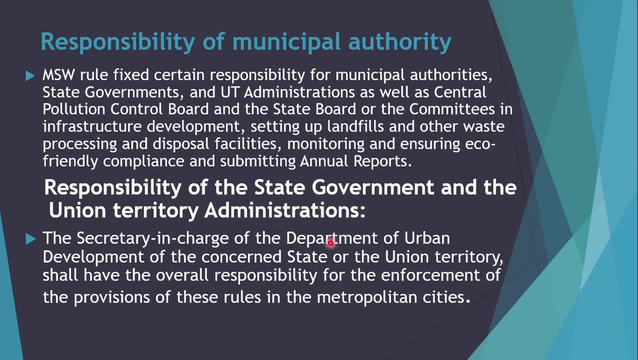 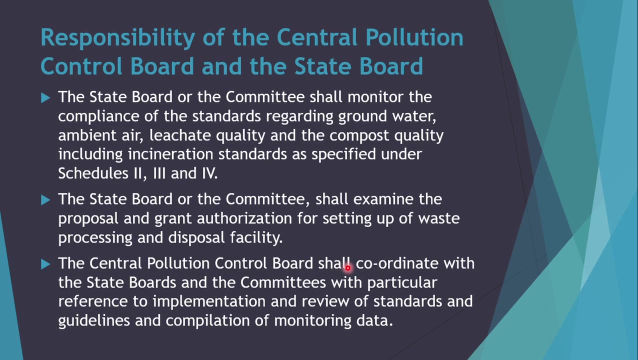 Responsibility of the State Government and the Indian Territory Administration. The Secretary in charge of the Department of Urban Development of the concerned State or the Union Territory shall have the overall responsibility for the enforcement of the provisions of these rules in the metropolitan cities, Coming to the Responsibilities of the Central and State Pollution Control Boards. 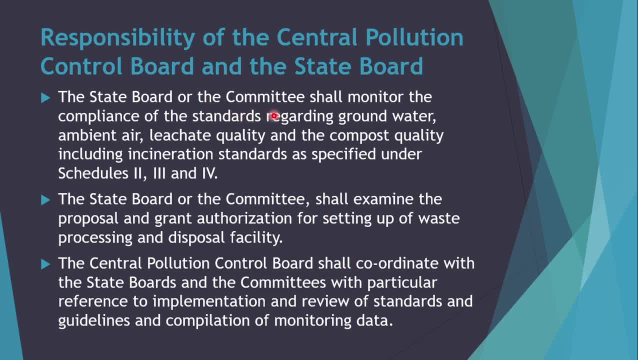 The State Board or the Committee shall monitor the compliance of the standards regarding groundwater and the ambient air quality and leakage quality near the landfill area and the compost quality, including incineration standards as specified under Schedule 2, Schedule 3 and Schedule 4.. 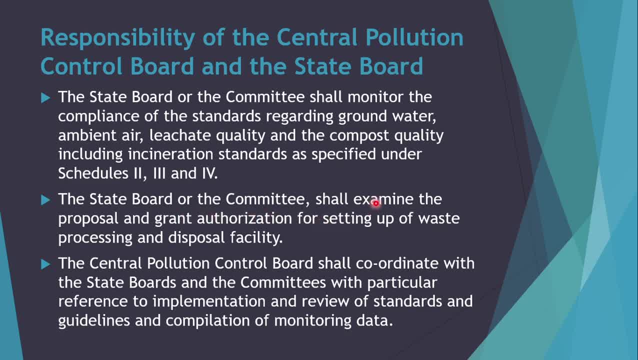 The State Board or the Committee shall examine the proposal and grant authorization for setting up of waste processing and disposal facility. Thank you, Coming to the Central Pollution Control Board. Central Pollution Control Board will coordinate with all the State Boards and the Committees with particular reference to implementation and review of standards and the guidelines prescribed by the CPCB. 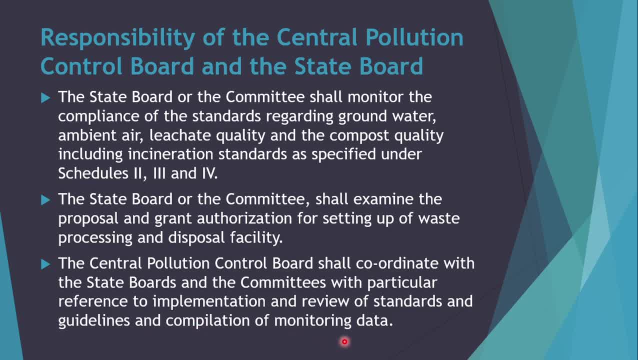 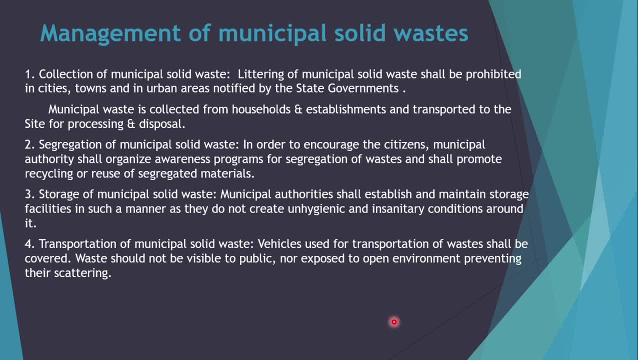 and compilation of all the monitoring data is done by Central Pollution Control Board. Central Pollution Control Board will be kimchi Management. Management of Municipal Solid Waste. It is done in various孩 and transported to the site for processing and disposal. 2. Segregation of municipal solid waste. 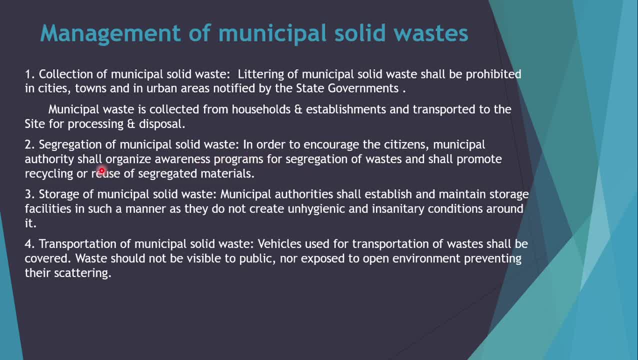 In order to encourage the citizens, municipal authorities shall organize awareness programs for segregation of waste and shall promote recycling or reuse of segregated materials. 3. Storage of municipal solid waste. Municipal authorities shall establish and maintain storage facilities in such a manner as they do not create unhygienic and insanitary conditions around it. 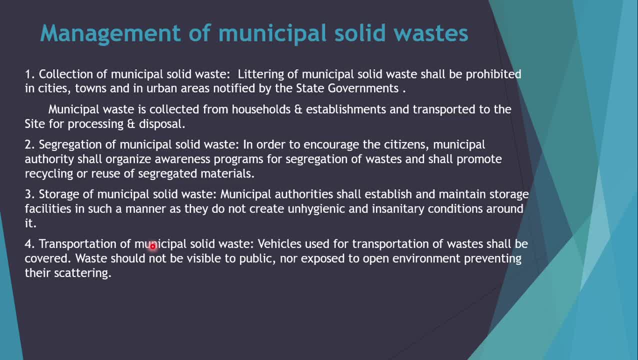 4. Transportation of municipal solid waste. Vehicles used for transportation of waste shall be covered. Waste should not be visible to the public. If they are transported on the road, they will be covered. If the public are moving, it is totally covered. 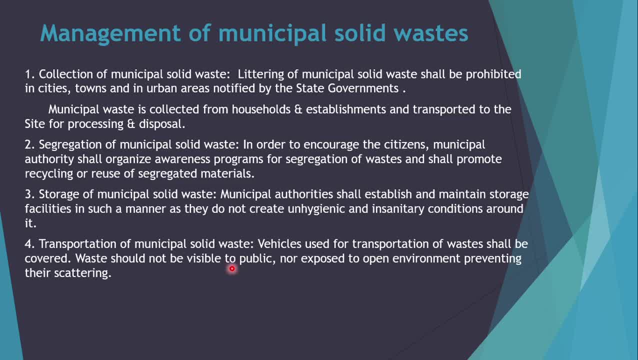 No leakage from that vehicle, No rusting is identified in that vehicle And properly painted vehicles they have to use And it is not visible nor exposed to the open environment, preventing their scattering. All these should be taken care by the municipal authorities. 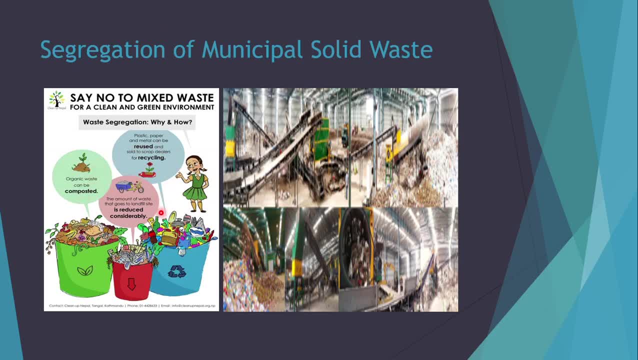 So segregation of municipal solid waste. Municipal solid waste will be done in the source, that means in the house itself. green, organic- that means organic waste- can be thrown in the green bin and whatever is recyclable- plastic paper- can be thrown in the blue and which used to throw in the landfill area can be reduced by segregating it in various forms. 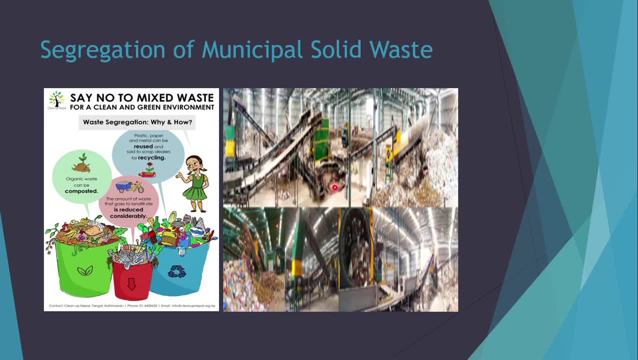 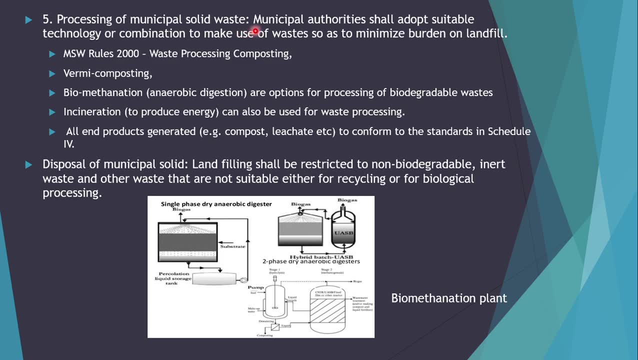 Using machines, we can segregate. we can segregate the municipal waste, Munефal Solid Waste. 5. Processing of municipal solid waste. Municipal authorities shall adopt suitable technology or combination to make use of waste so as to minimize burden on landfill area. 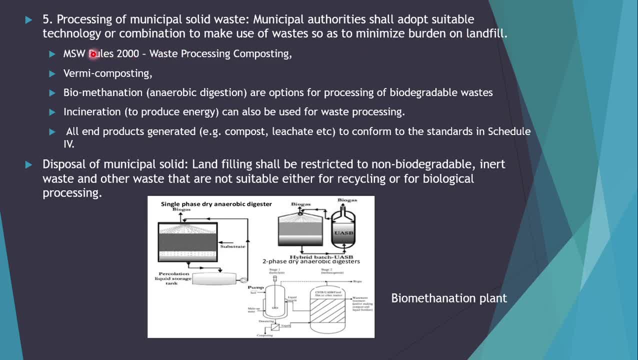 Munefal Solid Waste In 2000 rule processing and composting is done Vermicomposting using earthworms. when propagating haiathan Using earthworm, we can convert biodegradable waste into vermicompost. and biodegradable waste can be used to generate methane gas by the process of biomethanation, where the degradation is done in absence of oxygen. 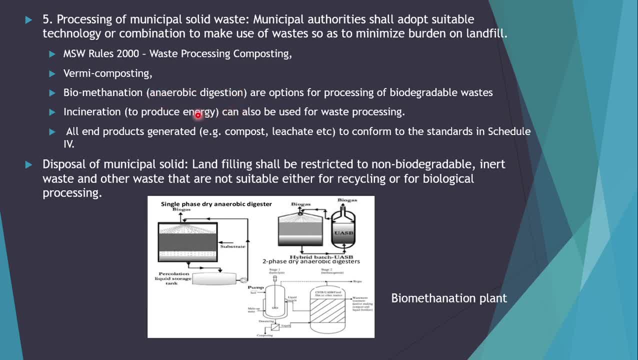 So it is called anaerobic digestion And next incineration to produce energy. Waste to energy we are hearing in these days. Incineration is by burning We can generate energy. All end products generated to conform to the standards in Schedule 4.. 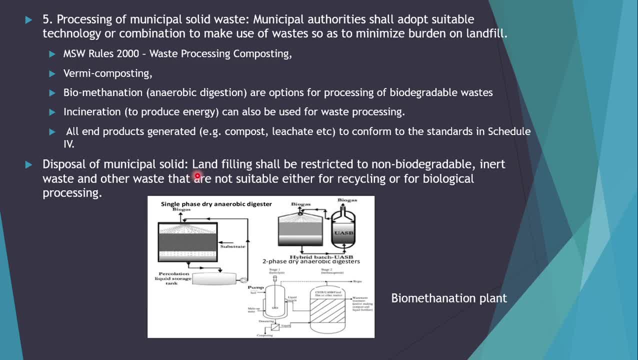 Last one, disposal of municipal solid waste Landfill area shall be restricted to non-biodegradable waste And other waste that are not suitable either for recycling or for biological processing. Here in this picture, you can see the biomethanation plants- Various biomethanation plants where the methane gas is generated from biodegradable waste. 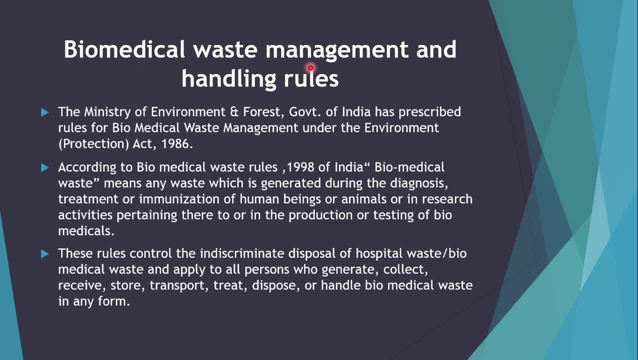 Coming to the next rule, biomedical waste management and handling rule. The Ministry of Environment and Forestry Government of India has prescribed this rule. The Ministry of Environment and Forestry has prescribed rules for biomedical waste management under the Environment Protection Act 1986. 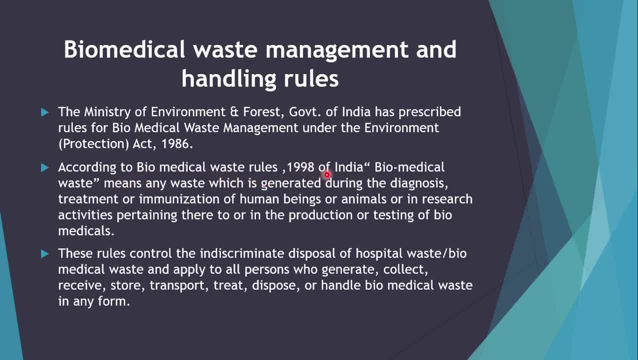 According to the Biomedical Waste Rule 1998 of India, biomedical waste means any waste which is generated during the diagnosis of any disease or during the treatment or immunization of human beings or animals, or in research activities. These are the activities pertaining there to or in the production or testing of biomedicals. 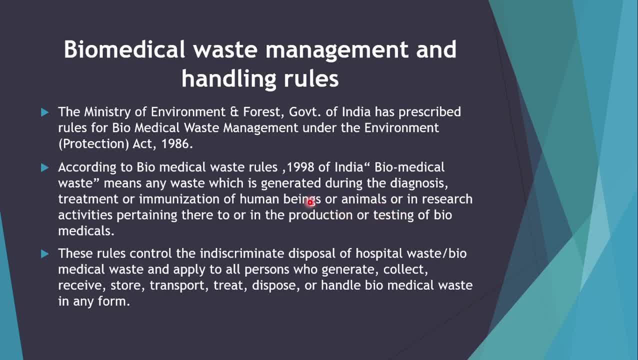 In all these areas and during all these processes, whatever is generated that can be considered as biomedical waste. These rules control the indiscriminate disposal of hospital waste or biomedical waste and apply to all persons who generate, collect, receive, store, transport and manage. 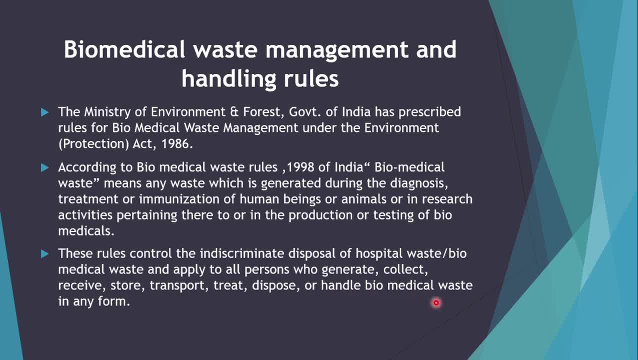 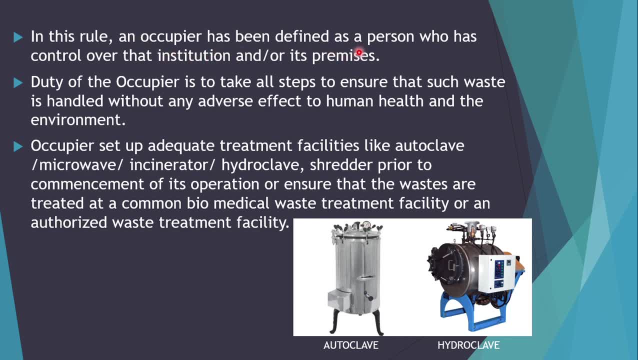 treat or dispose or handle biomedical waste in any form. In this rule, an occupier has been defined as a person who has control over that institution or its premises. Duty of the occupier is to take all steps to ensure that such waste is handled without any adverse effect to human health and the environment. 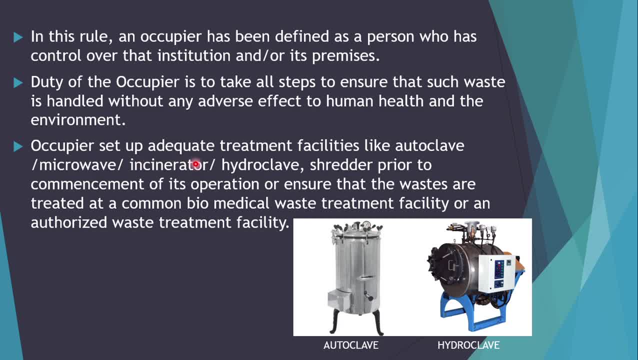 Occupier setup Adequate treatment facilities like autoclave. here you can see the picture of autoclave microwave incinerator. it is nothing but burning till ash or form hydroclaves where the liquid wastes are disinfected. here 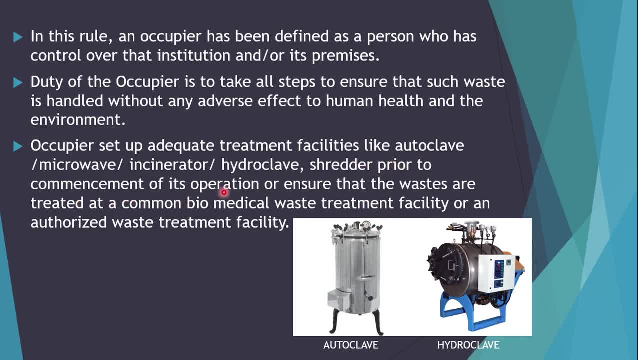 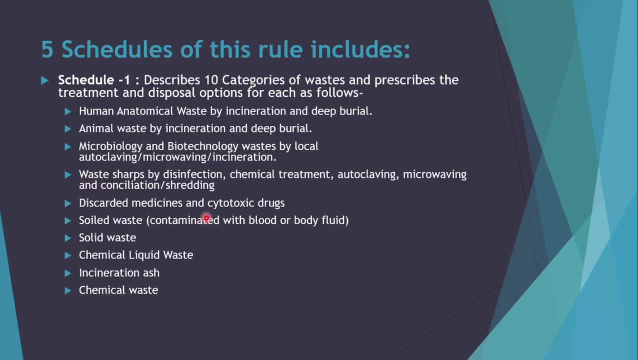 shredder, prior to commencement of its operation, are ensured that the wastes are treated at a common biomedical waste treatment facility or an authorized waste treatment facility. 5 schedules of this rule includes: Schedule 1 describes 10 categories of waste and prescribes the treatment and disposal options for each as follows. Under this: 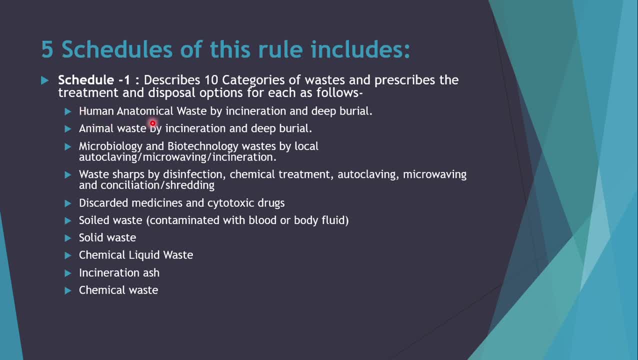 Schedule 1, first category is the waste disposal and disposal of waste, If you are. category means human anatomical waste. it has to be incinerated or deep buried in the soil. anatomical means: we all know cells are tissues from the human animal waste. second category comes 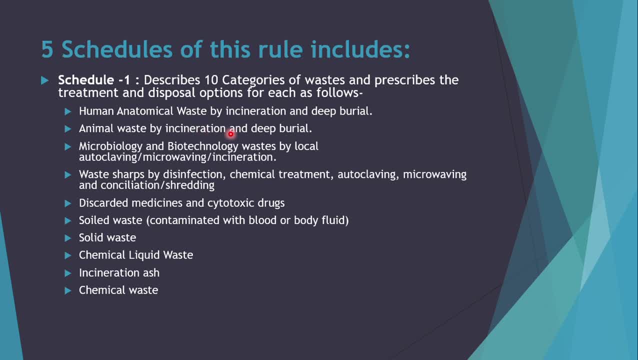 in animal waste. this also has to be incinerated or deep buried. next third category: microbiology and biotechnology waste. this can be autoclaved or microwaved or burnt till rashes are formed. that is incineration. fourth category: waste sharps. sharp means scalpels, forces, all these things. 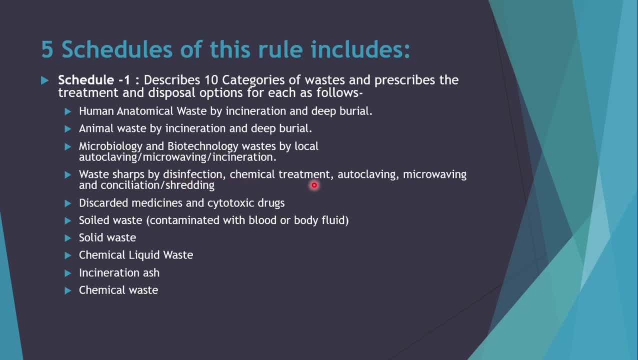 this can be disinfected by chemical treatment, using some chemicals, or they can be autoclaved or microwaved and conciliation or shredding. next fifth category will be discarded medicine and cytotoxic drugs. sixth category: soiled waste which is contaminated with blood or body fluids. seventh category: solid waste. eighth: chemical liquid waste. 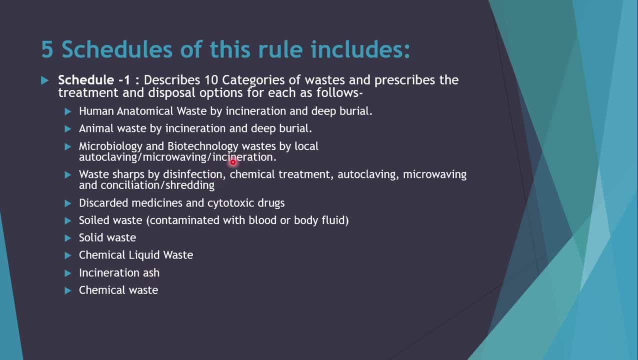 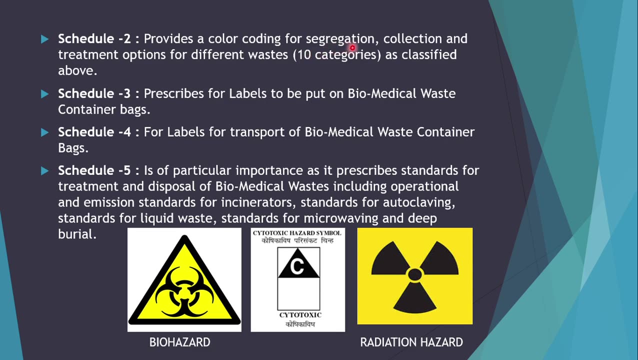 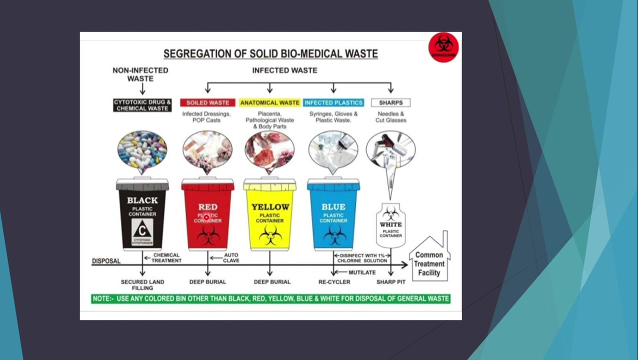 ninth, incineration ash. when we are burning here any waste, the ash which is generated is considered as ninth category. tenth one: chemical waste is consortium of shrapnel and vogel and polyester- now google bins or plastic covers where they are used to segregate this waste- cytotoxic. 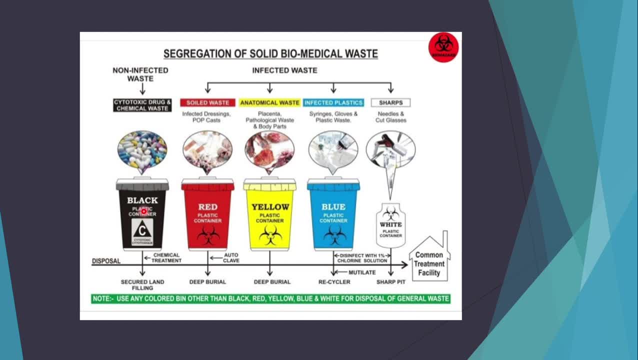 drugs and chemical waste are thrown in the black. one. soiled waste, infected dressings and other things are thrown in the red. one. anatomical waste are thrown in the yellow here syringes, gloves, plastic, all these are thrown in the blue. needles are cut, glasses or sharps are thrown in the white. all these are. 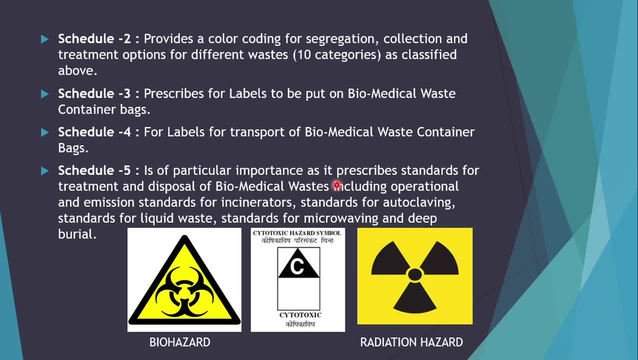 different colored containers where we have to segregate the biomedical waste and to discard schedule 3 prescribed for labels to be put on biomedical waste container bags. these are the few labels. where we are using biohazard waste is indicated in this manner. eccentrics are spit out, obstacles symbol is indicated, the radiation has. 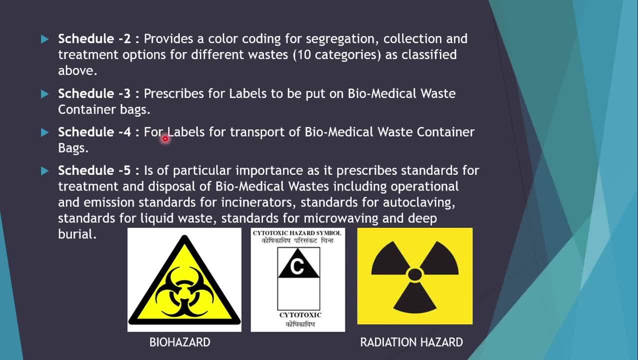 not symbol, is indicated and schedule for or labels were transport of biomedical waste container bags. schedule 5 is of particular importance and it describes standards for treatment and dispose the biomedical waste, including operational and emission standards for incinerators, standards for auto clearing, standards for liquid waste. 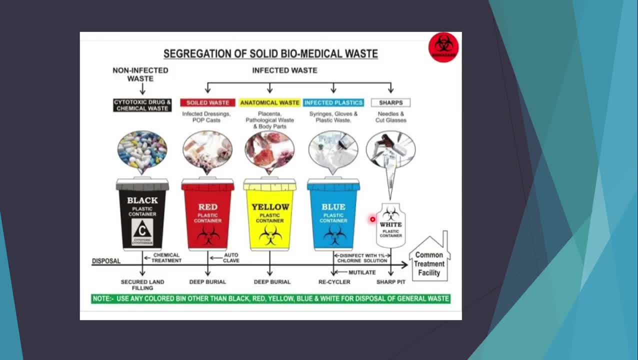 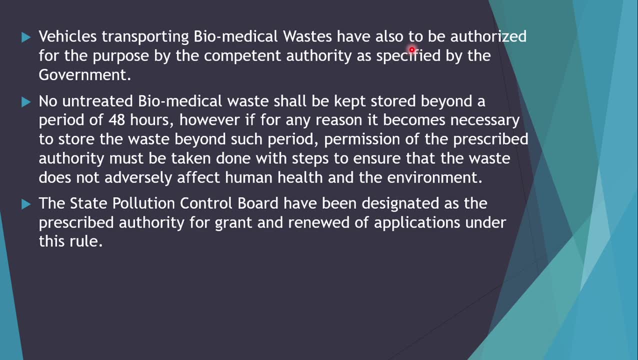 for microwaving in deep burial. vehicles transporting biomedical waste have also to be authorized for the purpose by the competent authority, as prescribed by the government. no untreated biomedical waste shall be kept stored beyond a period of 48 hours. however, if, for any reason, if an occupier has to store, it becomes. 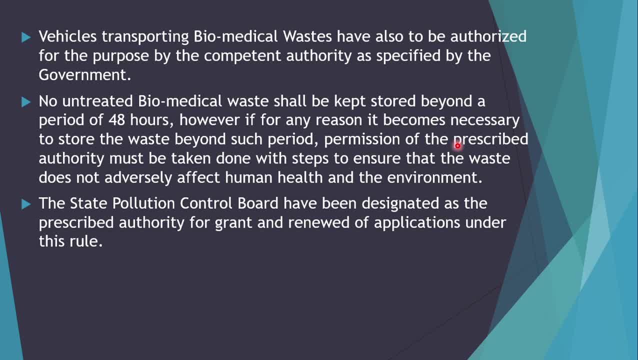 necessary to store the waste beyond such period he has to take. the prior permission from the prescribed authority must be taken done with steps to ensure that the waste does not adversely affect any human health in the environment, if at all. he has to store the waste beyond the 48 hours the state pollution control. 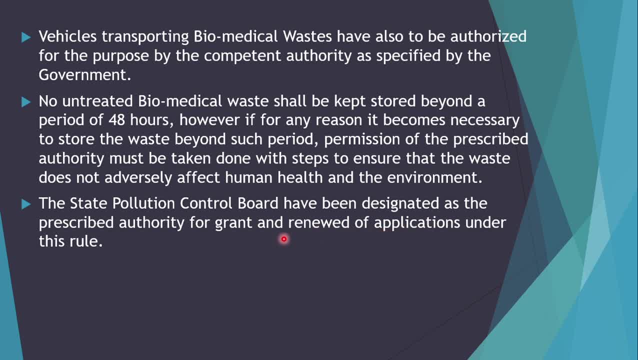 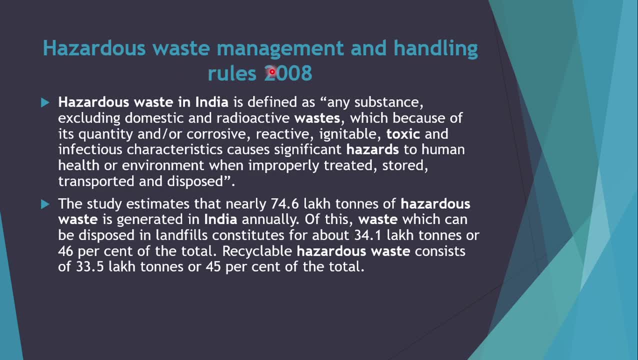 board have been designated as a prescribed authority for grant and renewal of applications under this rule. third rule: hazardous waste management and handling- rule 2008. hazardous waste in India is defined: defined as any substance, excluding domestic and radioactive waste, which, because of its quantity, or corrosive or reactive or 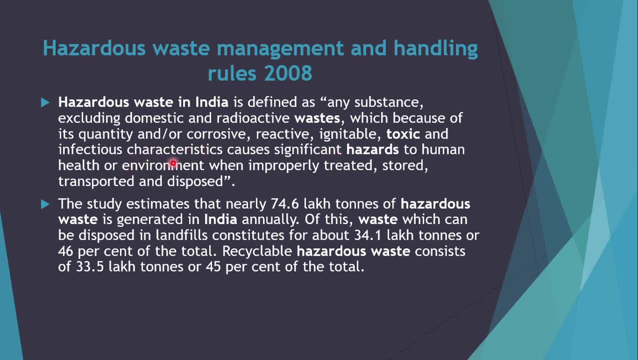 ignitable, toxic and infectious characteristics causes significant hazard to human health or environment when improper treated, stored or transported and disposed. the study estimates that nearly 74.6 lakh tons of hazardous waste is generated in India annually. of this, waste which can be disposed in landfills constitute about 34.1 lakh tons. it comes 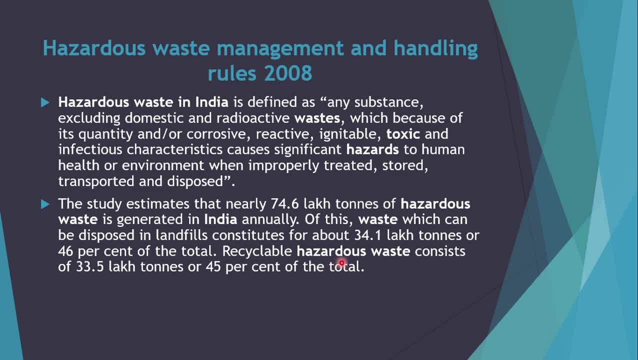 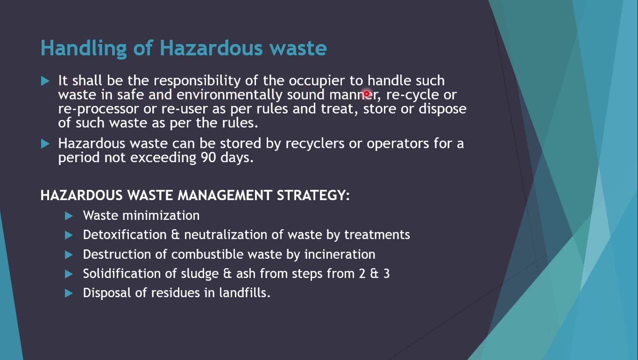 to 46 percent of the total waste, and recyclable hazardous waste consists of thirty three point five lakh tons, or it comes up to forty five percent of the total hazardous waste. Handling of hazardous waste: It shall be the responsibility of the occupier to handle such waste in safe and environmentally sound manner, Recycle or 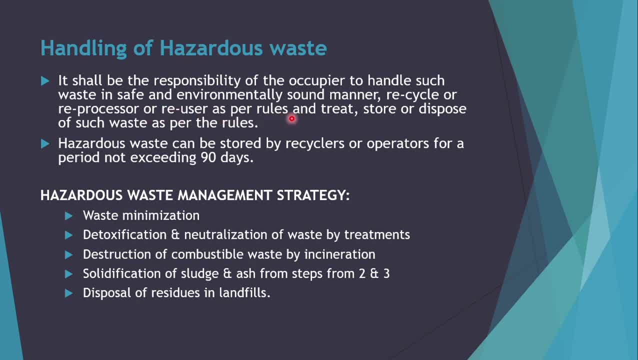 reprocessing or re-user as per rules, and treating the waste and storing it or dispose of such waste. as per the rules, Hazardous waste can be stored by recycler or operator for a period not exceeding 90 days. What are the strategies followed for hazardous waste management? 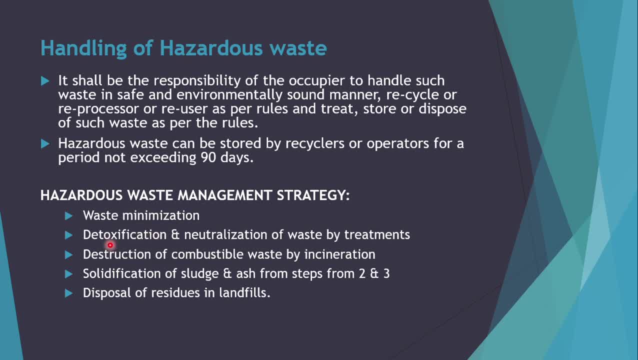 First one: waste minimization. Second one: detoxification or neutralization of the waste by treating the hazardous waste. Destruction of combustible waste by incineration. If it is possible for us to burn it till the ash is gone, we will follow incineration process. 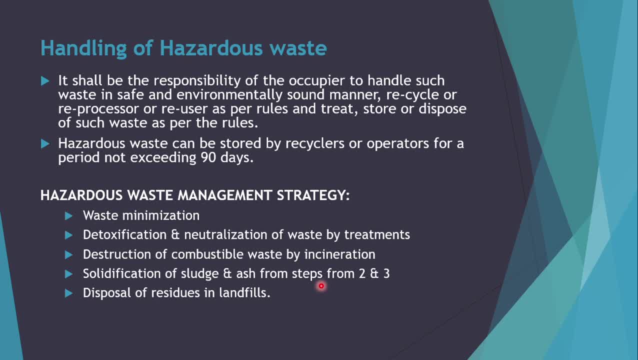 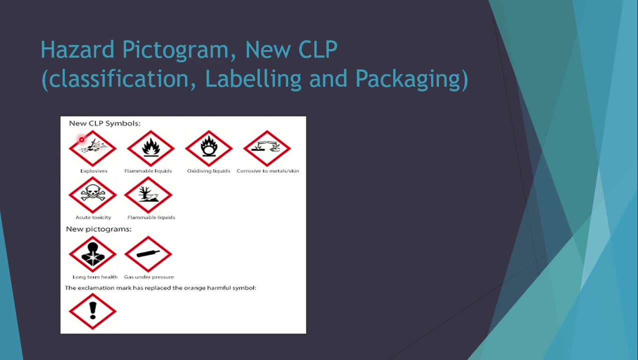 Next, solidification of sludge or ash, Some steps, that is here, from detoxification and the incineration. Disposable, disposal of residues in landfill area. Hazard pictograms and a new one, New CLP means. CLP stands for classification, labeling and packaging. 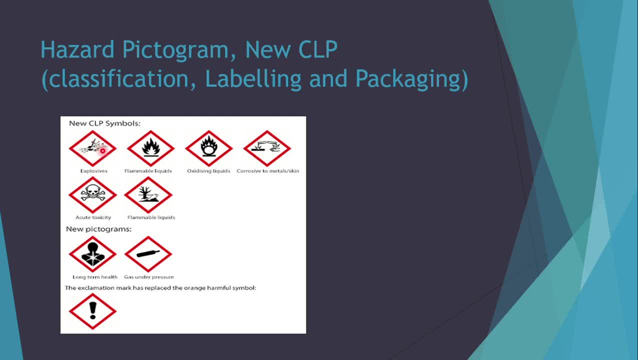 Explosive will be indicated in this form. Inflammable liquids are indicated in this form. Oxidizing liquids Corrosive to metals and skin is indicated in this symbol. Acute toxicity- if it is so toxic it is indicated in this symbol. Flammable liquids is indicated. 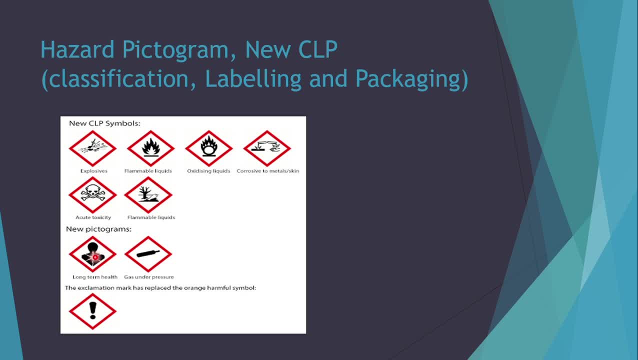 with this symbol. If any chemical has long-term effect on health, it is indicated in this symbol. gas, if it is under pressure, it is indicated with this symbol. so all these are various symbols used on the hazardous chemicals, export and import of hazardous waste. the Ministry of 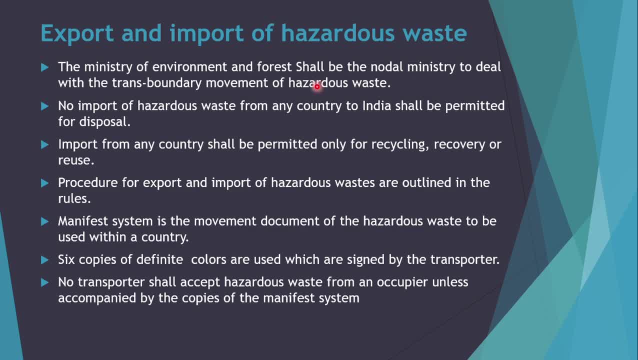 Environment and Forest shall be the nodal ministry to deal with the trans boundary movement and trans boundary means. export and import of hazardous waste. no import of hazardous waste from any country to India shall be permitted for disposal. import from any country shall be permitted only for recycling. 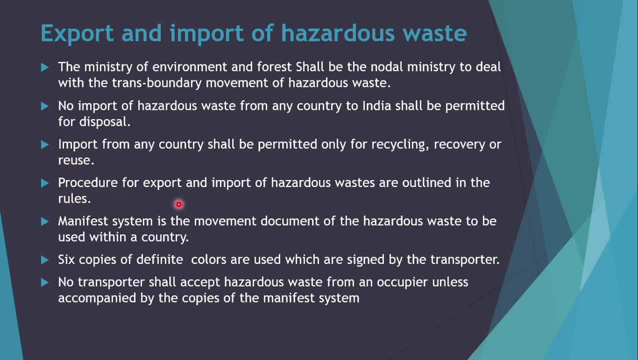 recovery or reuse procedure for export and import of hazardous waste are outlined. it rules. a manifest system is a smaller for the movement of the chemicals in the country, so that manifest system is a movement document of that waste to be used within a country. In this six copies of definite colors are. 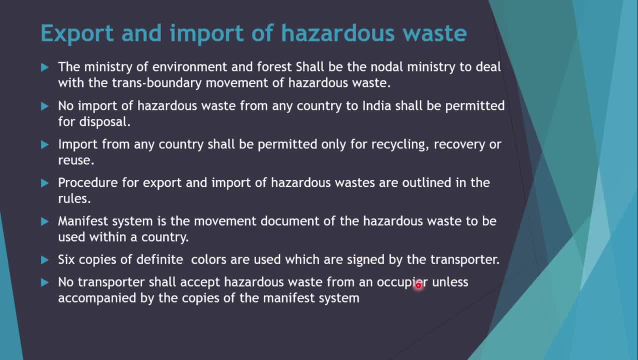 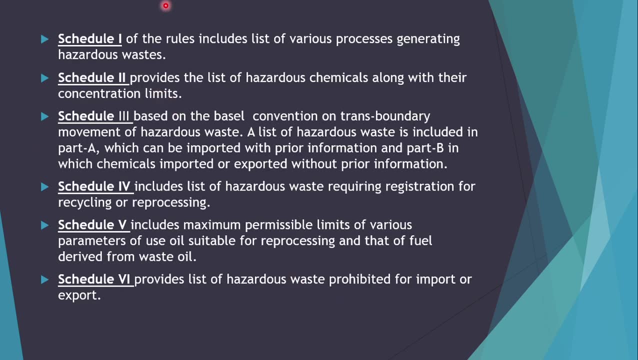 used which are signed by the transporter, and no transporter will accept this hazardous waste from an occupier unless it contains these manifest system copies. Schedule one of this hazardous waste management rule includes list of various processes generating hazardous waste In the schedule 2 provides the list of: 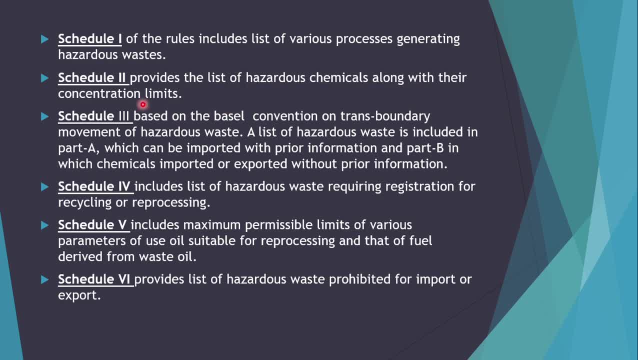 hazardous chemicals, along with their concentration limits. In schedule 3, based on the basal convention on transboundary movement of hazardous waste, A list of hazardous waste is included in part which can be imported with prior information and in part The chemicals which can be imported or exported without any prior information. In Schedule 4, it includes a list of hazardous waste requiring registration for recycling or reprocessing. 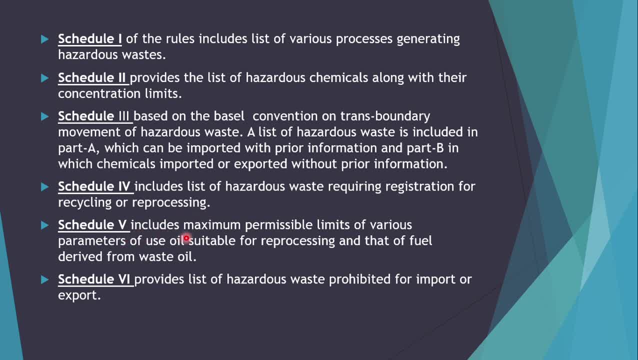 Schedule 5 of hazardous waste management includes maximum permissible limits of various parameters of used oil suitable for pre-processing and that of fuel derived from waste oil. Schedule 6 provides a list of the hazardous waste prohibited for import or export. Treating hazardous waste by chemical thermodynamics. 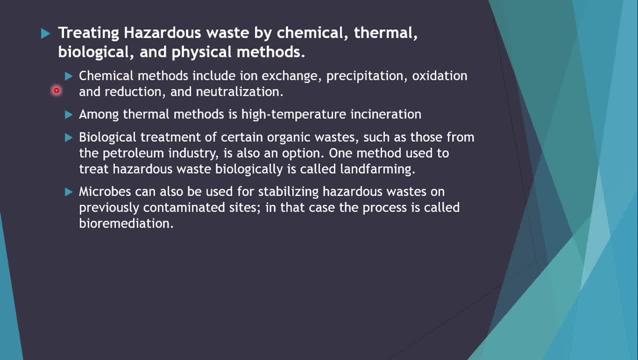 The hazardous waste can be treated by various following methods. Chemical methods include ion exchange process, precipitation, oxidation, reduction and neutralization. These are the methods used for treating the hazardous waste. Thermal methods include high temperature incineration. If you can burn the hazardous waste, then this method can be used. 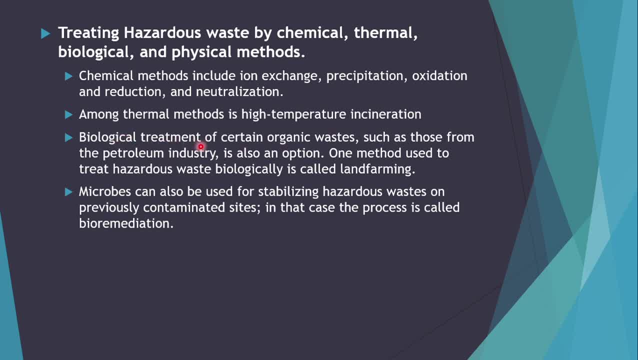 Biological treatment of certain organic waste. That means using some microbes we can treat the hazardous waste, such as those from the petroleum industry, And one method used here: using some microbes we can treat the hazardous waste. Then microbes can also be used for stabilizing hazardous waste and previously contaminated sites, and in that case the process is called bioremediation. 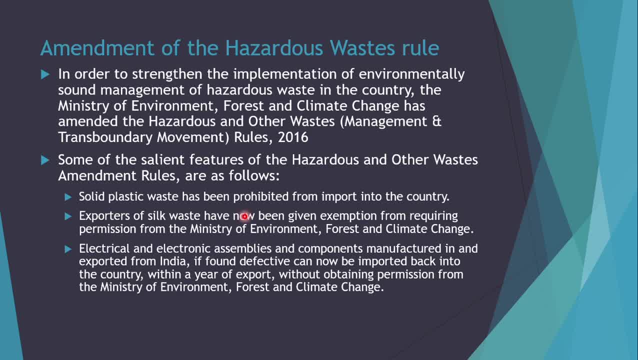 Amendment of the hazardous waste rule. In order to strengthen the implementation of environmentally sound management of hazardous waste in the country, the Ministry of Environment, Forest and Climate Change has amended the hazardous and other waste in 2016.. And some of the salient features are: solid plastic waste has been prohibited from import into the country.